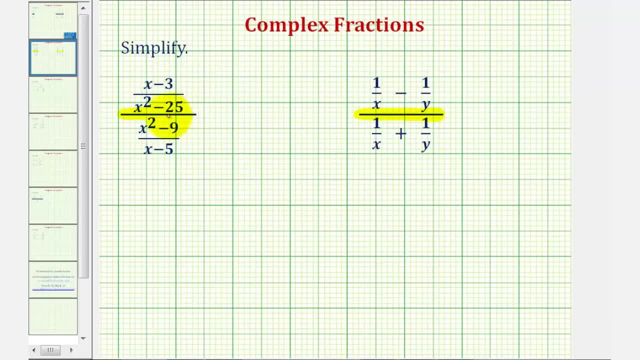 and a single fraction in the denominator and a fraction bar means division. we can write this as a division problem. This is equivalent to the quantity x minus three divided by the quantity x squared minus twenty-five divided by the fraction in the denominator. 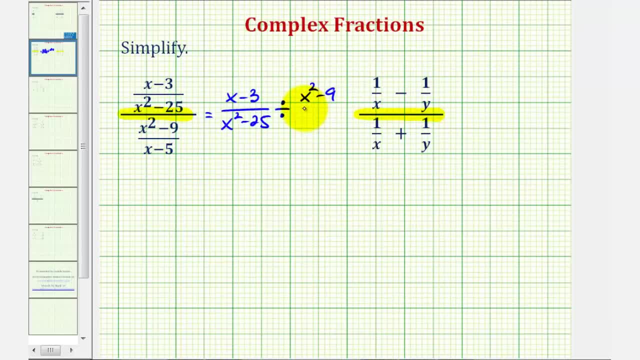 or the quantity x squared minus nine, divided by the quantity x minus five. Now we know, when dividing by fractions we normally multiply by the reciprocal instead. So we can write this division problem as a multiplication problem. So the first fraction will stay the same. 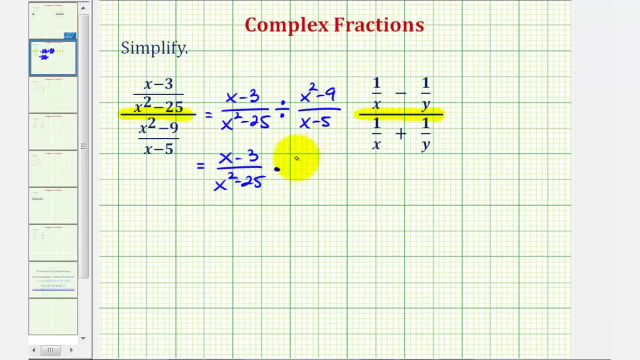 times the reciprocal of the second fraction, which would be the quantity x minus five divided by the quantity x squared minus nine. Now, before we multiply, we do want to simplify. To see what simplifies, we want to factor the numerators and denominators. 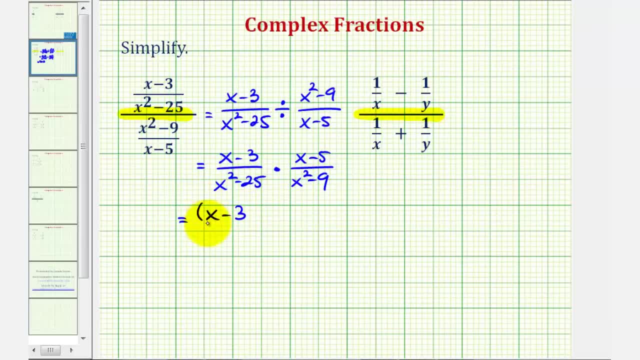 Well, the quantity x minus three doesn't factor, so we're going to divide by the number of fractions. but x squared minus twenty-five is a difference of squares, So we'll have x and x, and since five times five is equal to twenty-five, 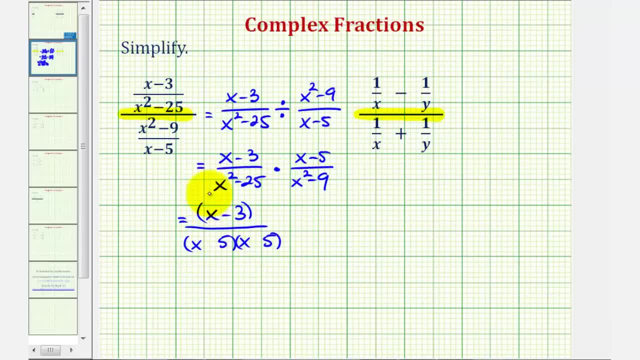 we'll have a factor of five here and a factor of five here, where one binomial is a sum and the other is a difference. And then times x minus five doesn't factor, but again, x squared minus nine is a difference of squares. 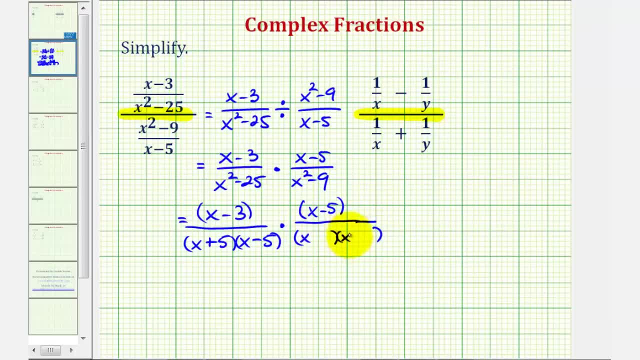 so we'll have two binomial factors, x and x, and since three times three is equal to nine, we'll have a factor of three here, a factor of three here, and one's a sum and one's a difference. Now we can see there are common factors between the. 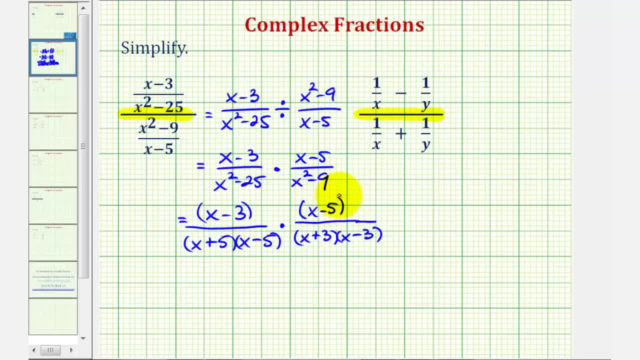 numerators and denominators that will simplify to one. Notice that x minus five over x minus five would simplify to one, and so would x minus three over x minus three. So now we're left with a numerator of one, and our denominator contains two factors. We have a factor of x plus five. 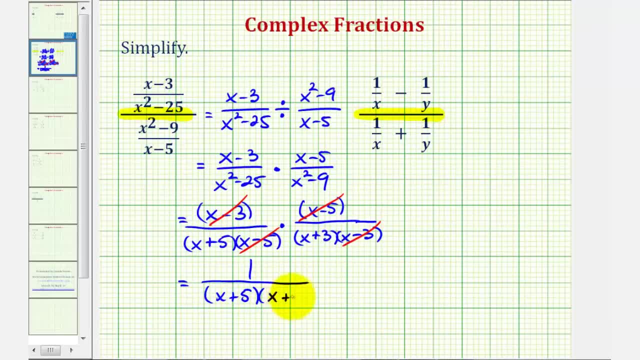 plus five and a factor of x plus three. This is the simplified form of the original complex fraction. Now, what's different about our second example is that we have a difference of two fractions in the numerator and a sum of two fractions in the denominator. 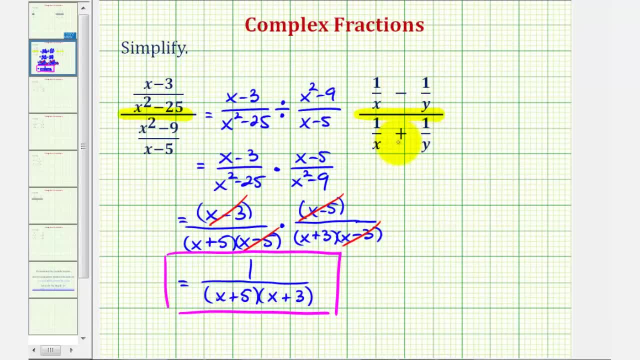 So we're going to find this difference and then find this sum before we write the division problem. And we know, in order to add fractions we must have a common denominator. so if we have a denominator of x and a denominator of y, the least common denominator would be x times y. 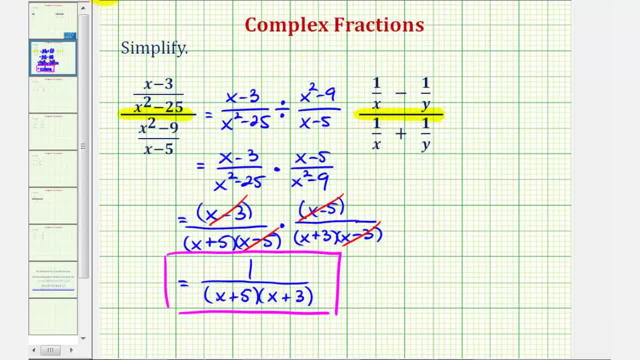 So if we want our denominators to be x times y or xy, we have to multiply one over x by y over y. Notice how our denominator is xy. and then for one over y, we have to multiply by x over x. Notice our denominators contain the same factors. 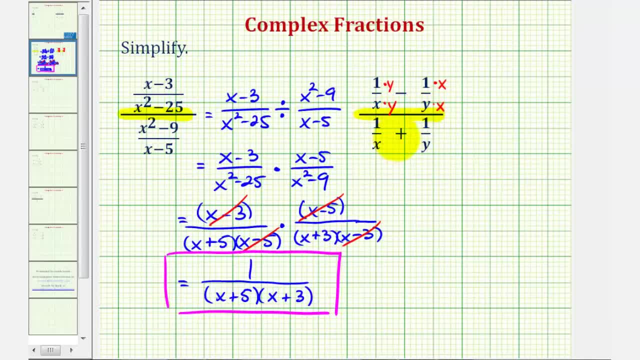 and therefore we have our common denominator. And to get the sum in the denominator, notice how the common denominator is also going to be xy. So multiply this first fraction by y over y and the second fraction by x over x. So now we have y over xy. 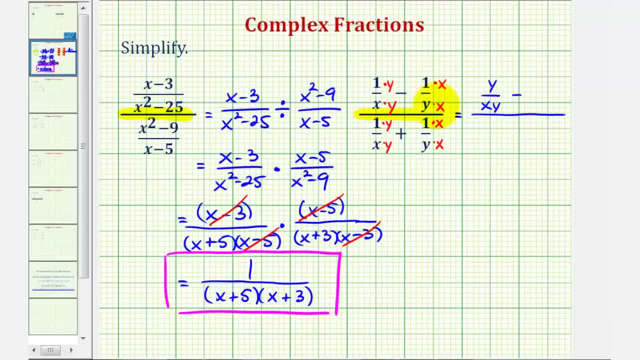 minus this would be x over yx or just xy. Remember we can change the order of multiplication without changing the product. And then for the sum below we have, we have y over xy plus x over yx or xy. 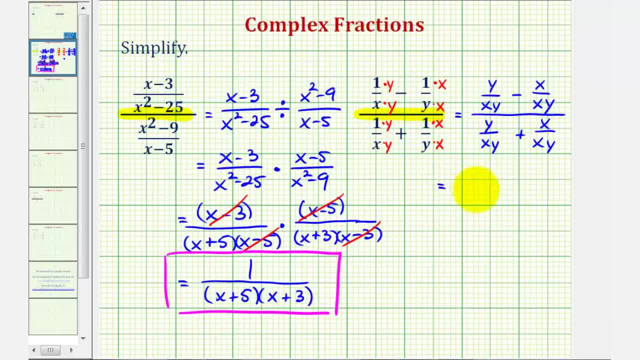 Now we'll go ahead and find this difference: in this sum, Common denominator of xy, the numerator would just be y minus x. And then for the sum below common denominator is xy and our numerator is y plus x. And again, remember this fraction: bar means division. 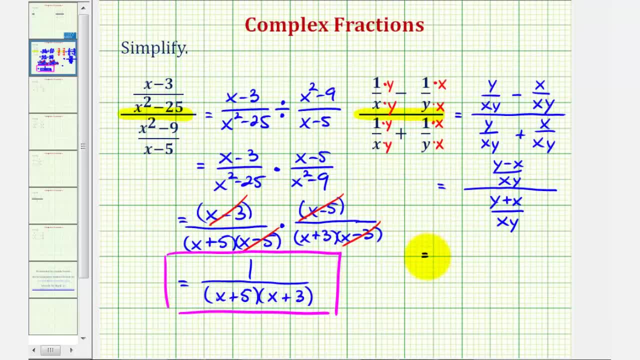 So let's go ahead and write this as a division problem. We would have y minus x divided by xy, divided by y plus x divided by xy. Now we'll go ahead and write this division problem as a multiplication problem, So we would have y minus x. 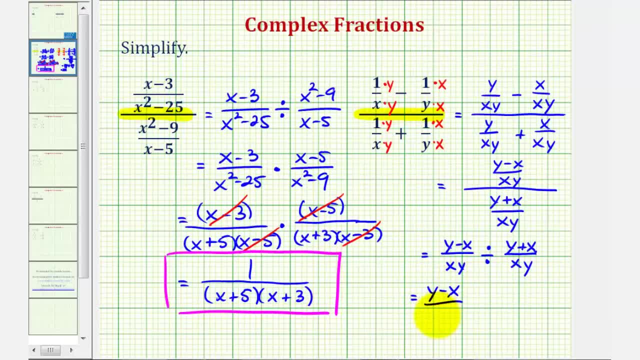 divided by xy. divided by xy, So we would have y minus x. divided by xy, So we would have y minus x, divided by xy times the reciprocal, which would be x times y times the reciprocal, which would be x times y. 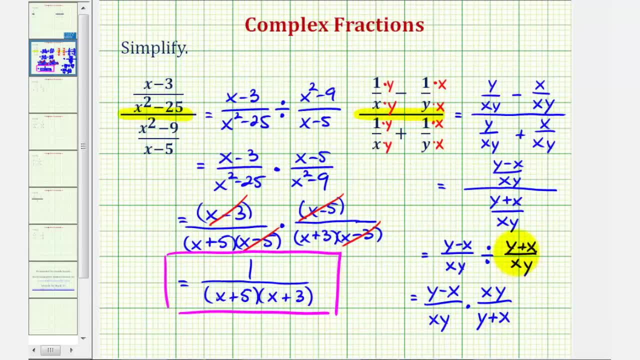 divided by the quantity y plus x. And notice: in this form this product will simplify. We have a factor of x over x that simplifies to one, and also a factor of y over y that simplifies to one. Notice: here we can't simplify because